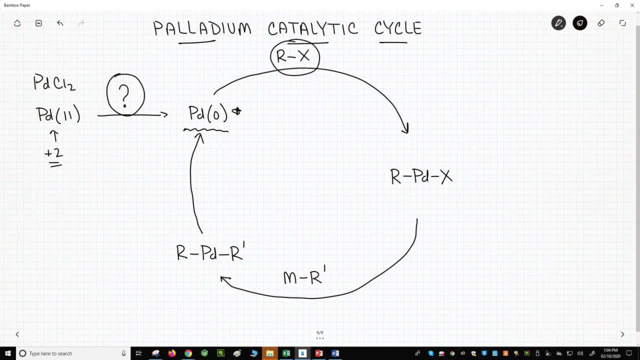 zero reacts with the aryl halide Rx to form an aryl-palladium halide, Rpdx. This reaction is called an oxidative addition. This may look strange, but if you've learned the Grignard reaction, you already know this reaction. Just like magnesium, zero can slide. 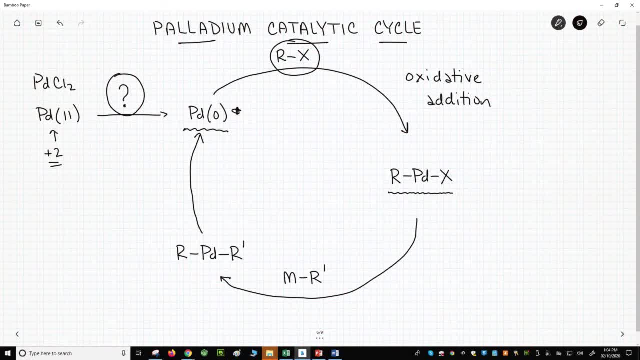 into a carbon-halogen bond to give a magnesium plus two complex palladium zero can do the same reaction to give a palladium plus two complex. The term oxidative refers to the oxidation state of palladium, which goes from zero to plus two. 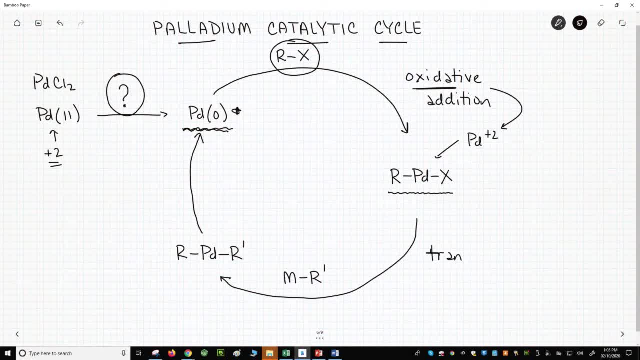 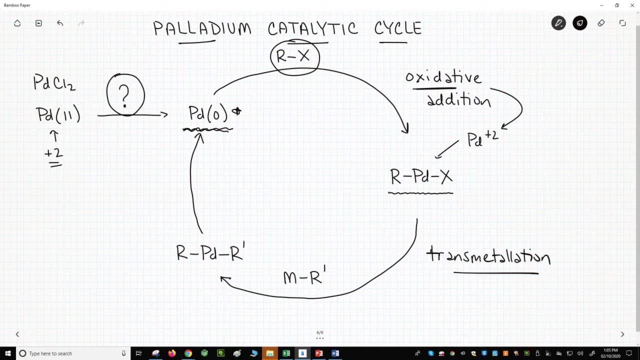 The next step is called a transmetallation. The aryl metal at the bottom – and let's think of this as an ionic species R'- metal plus – reacts with r-palladium-x to form r-palladium-r' as the new palladium species, and we lose. 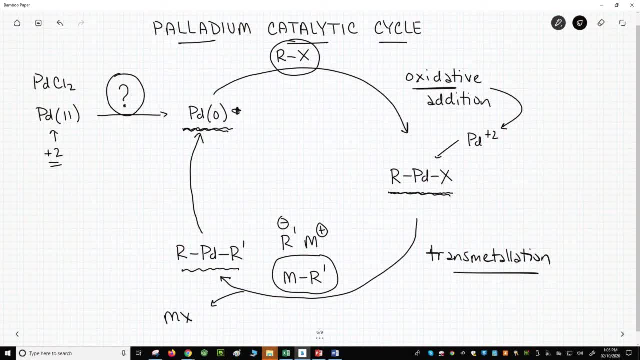 a metal halide salt. This is called a transmetallation because the R' group goes from having a bond from one metal, M, to having a bond to a different metal, palladium. Formally, palladium is still considered a radical charge. In this case r' helps with the plus two oxidation step. 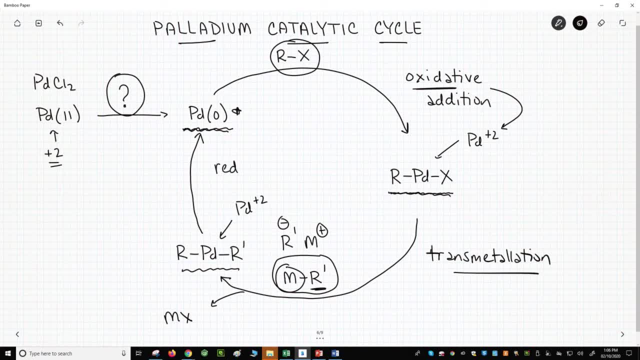 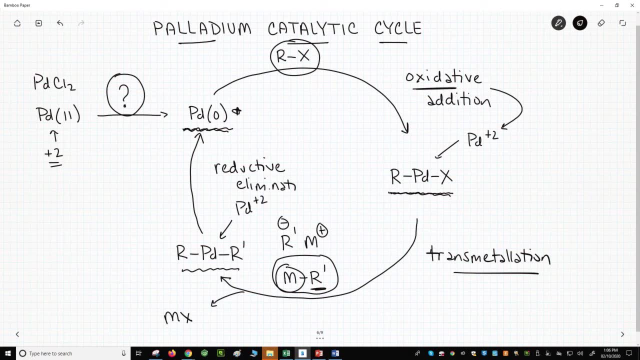 The final step is called a reductive elimination. Palladium, bound to what amounts to two carbon ions, R and R', is not very stable. The palladium slips from between the R and R' groups. Palladium is on the large side of the solid group and R is on the small side of the solid group. They can break down to different amigoids, Otherwise the r and they can still remain between each other. Then if you consider the r and r' groups as지고, they could also be a little bit more similar. As we started talking about the r and the r' groups, you'll see that the r and r groups are: